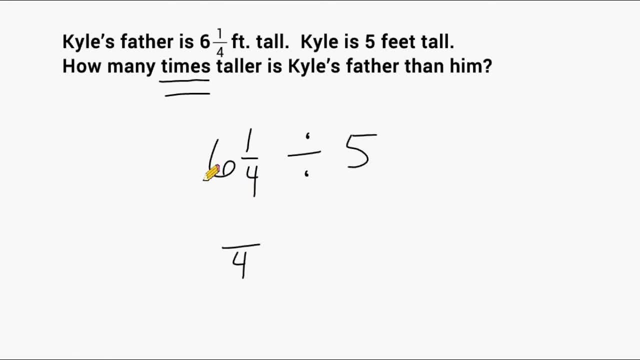 the denominator times a whole number. 4 times 6 is 24 plus our numerator is 25.. So 25 quarters is equivalent to 6 and 1 quarter And we have to change any whole numbers into a fraction, And when we are dealing with dividing fractions we have: 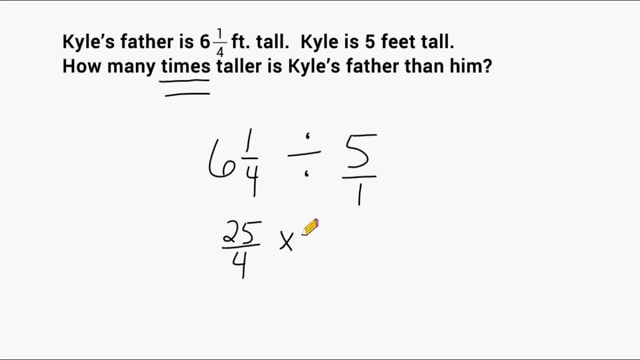 to change our division sign to multiplication and write the reciprocal of the second fraction. So now we have the fraction 25 quarters multiplied by 1. fifth Now, if we multiply 25 by 1, we get 25, and 4 times 5 is a product of 20.. 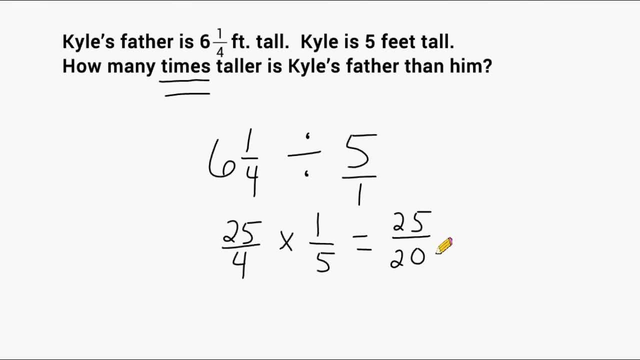 Now 25 and 20 both share a common factor of 5, so we can divide the top and the bottom numbers by 5 to reduce this fraction, And 25 divided by 5 is 5.. And 20 divided by 5 is 4.. 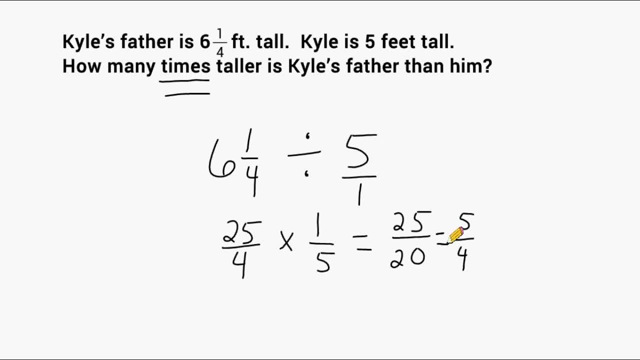 Now we can take our improper fraction of 5 quarters and rename that as a mixed number, And to do that you really just divide your numerator by the denominator. Well, 5 divided by 4 is 1, with 1 left over. 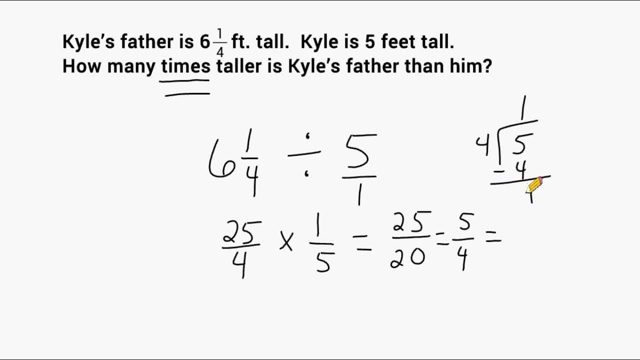 But that left over, we use to express as our numerator over a denominator. So we would say that 5 quarters is equivalent to 1 and 1 fourth. So we would say that Kyle's father is 1 and 1 fourth times taller than his son. 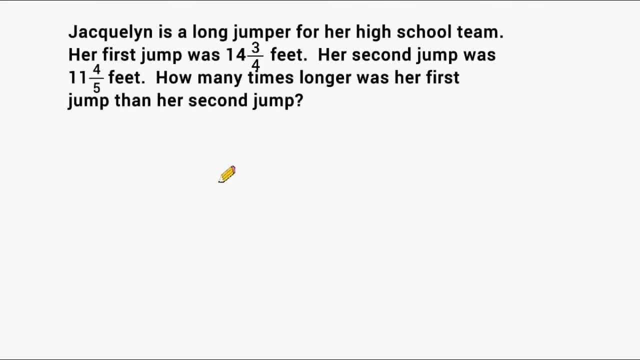 Okay, let's try another example. This problem reads that Jacqueline is a long jumper. for her high school team, Her first jump was 14 and 3 quarters feet, Her second jump was 14 and 3 quarters feet And her second jump was 11 and 4 fifths feet. 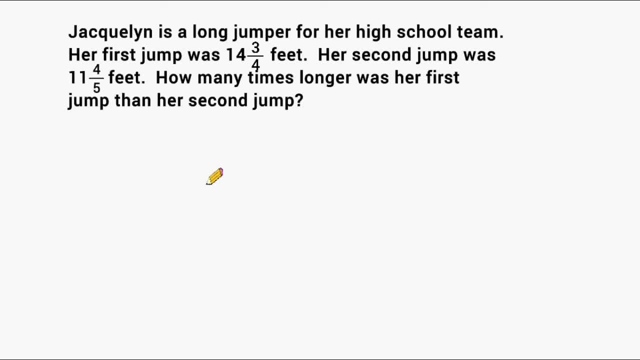 How many times longer was her first jump than her second jump? So we're going to start with the longer jump, which is 14 and 3 quarters feet, And we are going to divide that by the length of her second jump, which is 11 and 4 fifths feet.